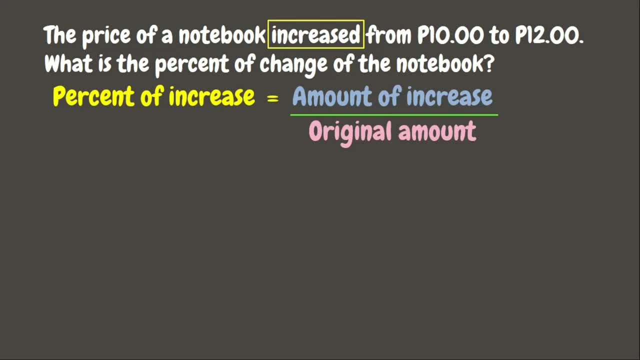 Wonderful. You are right. To get the amount of increase, we need to subtract the original amount from the new amount. This gives us our new formula, which is: Percent of increase equals new amount minus original amount, over or divided by the original amount. 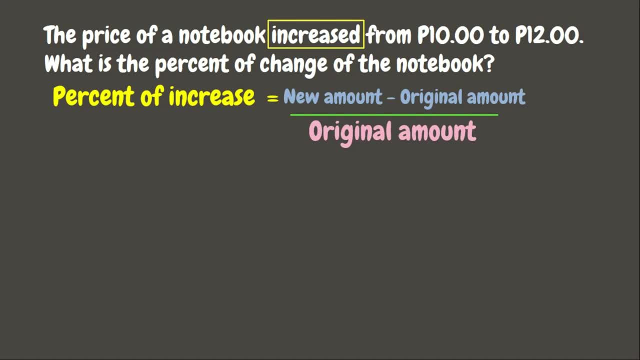 Now let us substitute the: given The new amount or the new price of a notebook is 12 pesos Minus the original amount, or the original price of a notebook, Which is 10 pesos Divided by the original amount, which is 10.. 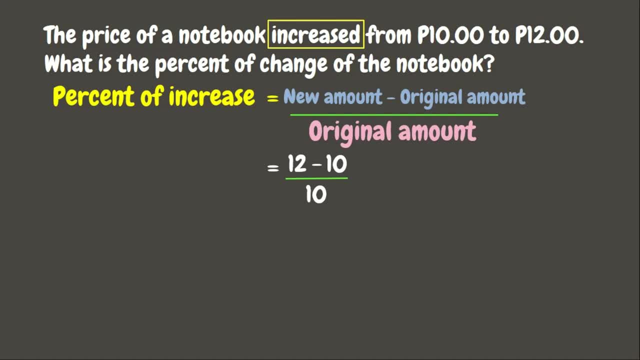 Now let us solve: 12 minus 10 is 2. Divided by 10.. Now let us divide 2 by 10.. 2 divided by 10.. 2 divided by 10.. 2 divided by 10.. 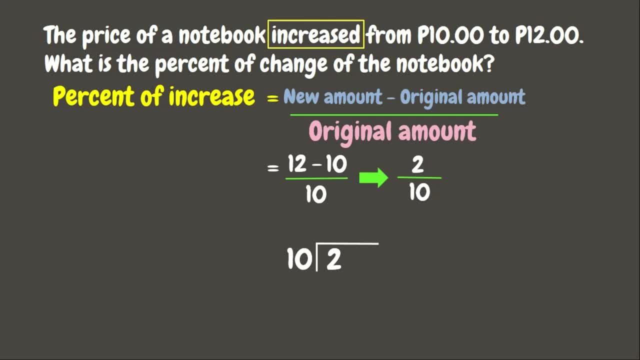 Since 2 is smaller than 10, let us add 0.0.. There, Let us put first the decimal point aligned from the decimal point in the dividend. There you go. Now. let us divide: 20 divided by 10 is 2.. 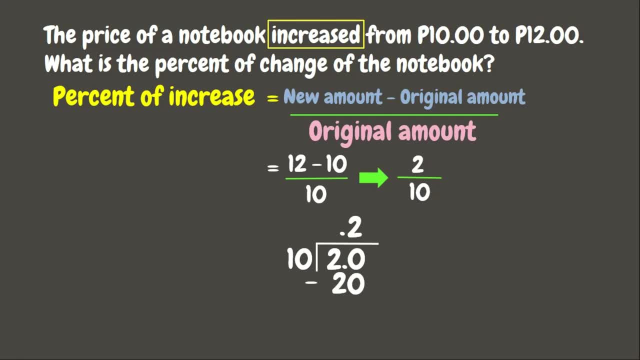 2 times 10 is 20.. 20 minus 20 is 20 minus 20 is 20 minus 20 is 0.. Our answer is 0.2. But since we are looking for the percent, we need to change the decimal into percent. 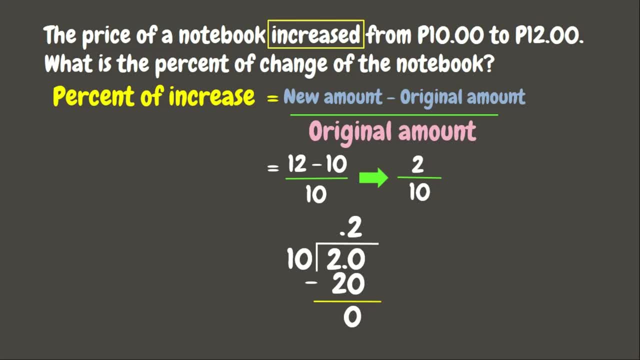 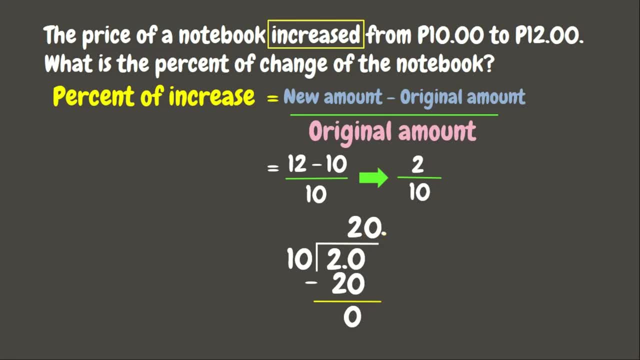 Let us put 0 to the empty place value And then change the decimal point into percent sign, And then change the decimal point into percent sign. Now our final answer is 20%. This means that the percent of change of the notebook is 20%. 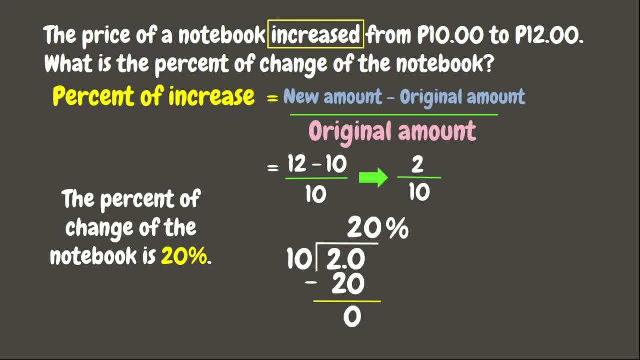 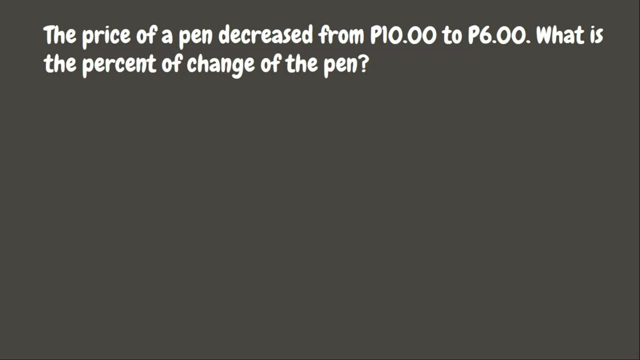 Wonderful. Now let us have another one. Let us try our second example. Let us try our second example. The price of a pen decreased from 10 pesos to 6 pesos. Now, what is the percent of change of the pen, Since we can see from the given situation that the price of pen decreased? it means 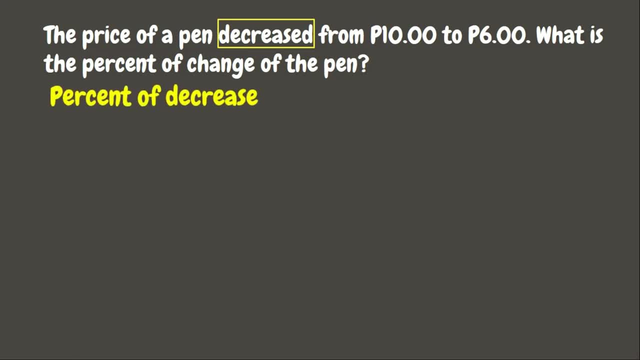 that we are looking for the percent of decrease Now. to get the percent of decrease, we need to divide the amount of decrease that we are looking for Now. to get the percent of decrease, we need to divide the amount of decrease that we are. 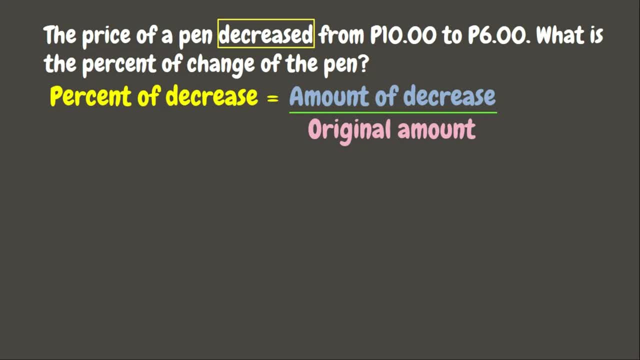 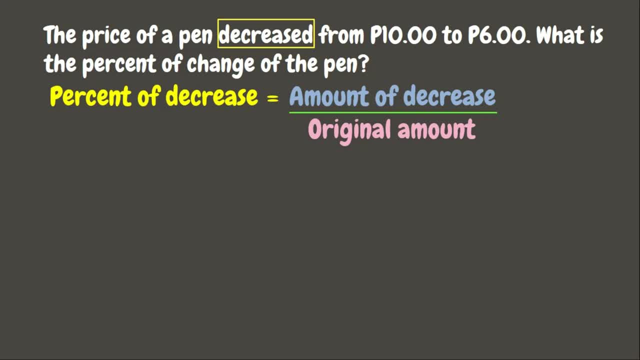 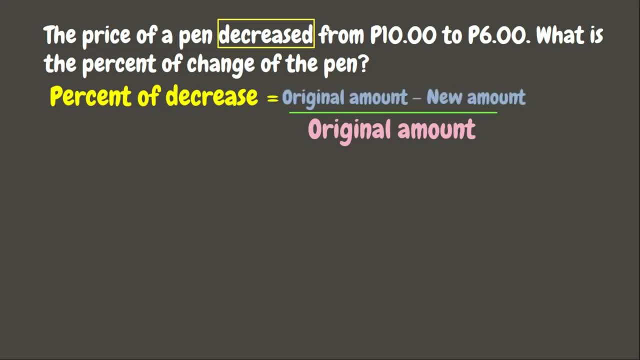 looking for Now to get the percent of decrease, we need to divide the amount of decrease that we are looking for amount from the original amount. let us write it down: the original amount or the original price of the pen is 10 pesos minus the new amount or the new price, which is 6 pesos over, or divided. 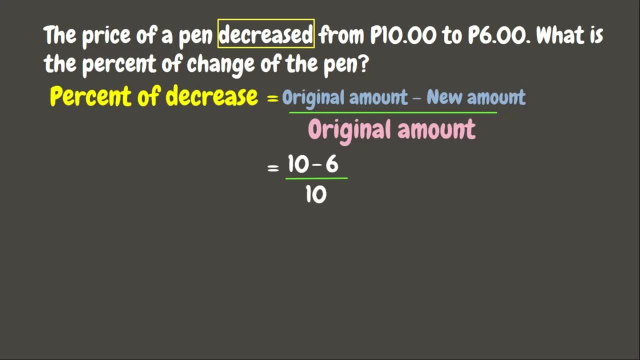 by the original amount, which is 10.. now let us solve: 10 minus 6. is 4 divided by 10.. let's divide 4 by 10.. since we know that 4 is smaller than 10, we need to add 0.0. there you go. 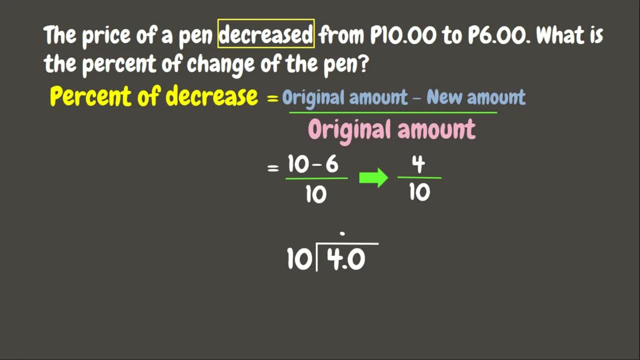 let's put first decimal point above. now let's divide: 40 divided by 10 is 4. 4 times 10 equals 40. now let's subtract, that gives us 0. now our answer is 0.4, but we need to convert it or change it into percent.